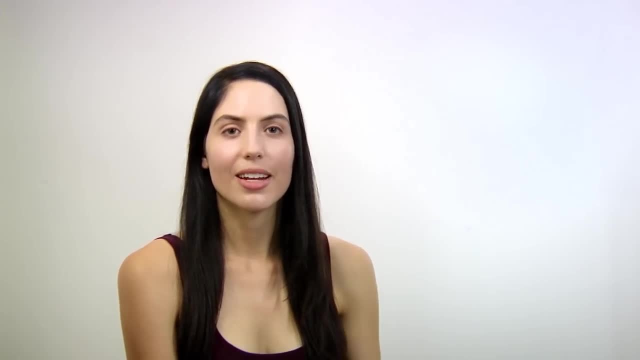 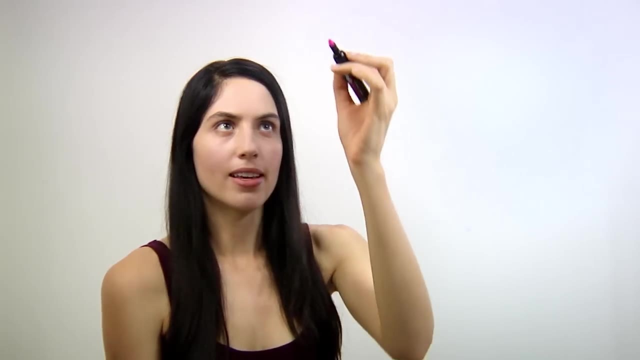 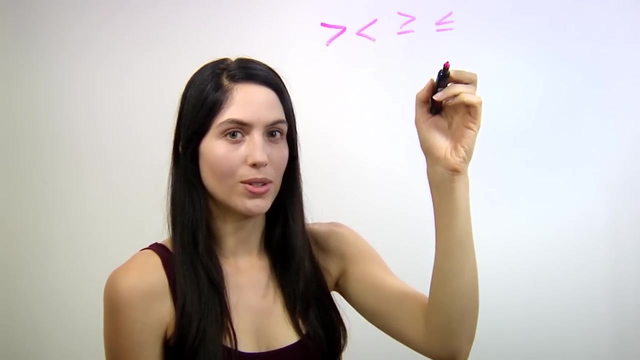 Hi guys, I'm Nancy and I'm going to show you how to solve an inequality. So an inequality is just any equation that has a greater than, less than greater than or equal to, or less than or equal to sign instead of the normal equal sign. In this video, we're going to focus 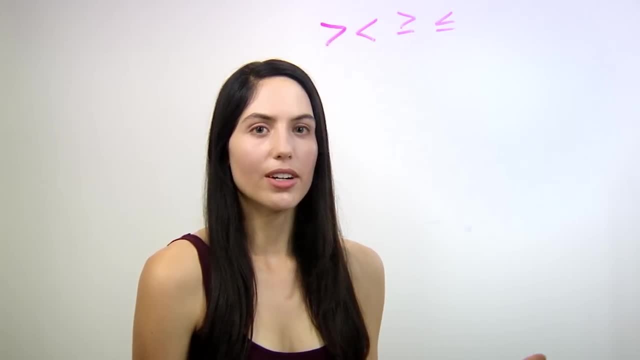 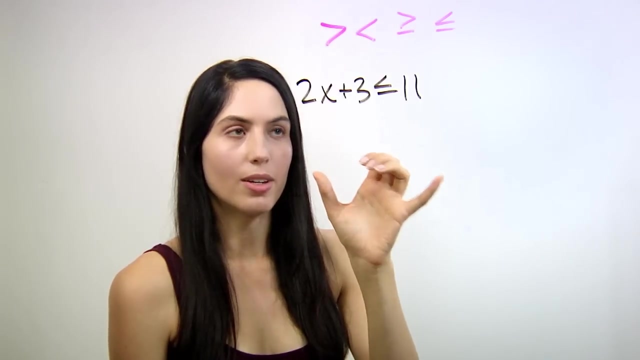 on linear inequalities. If you're looking for a quadratic inequality example, that's another video. If you don't know what I'm talking about, this is the right video for you. Here's a simple linear inequality example: 2x plus 3 is less than or equal to 11.. For 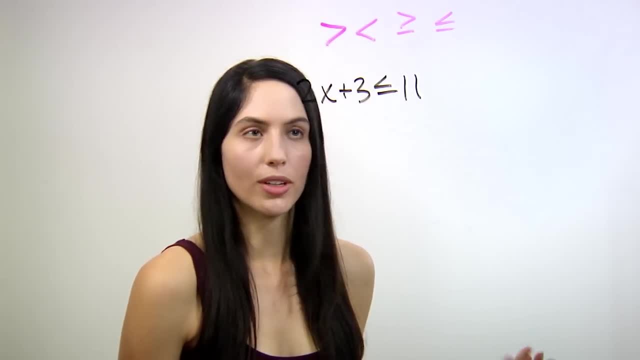 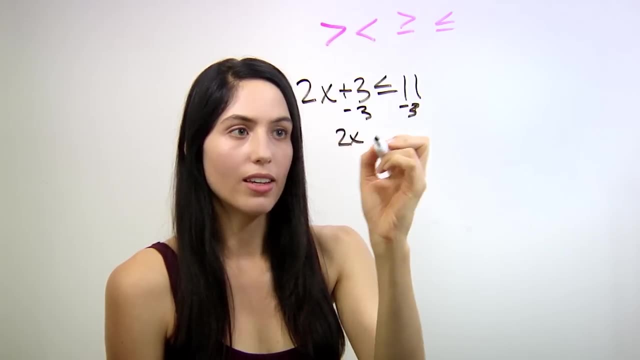 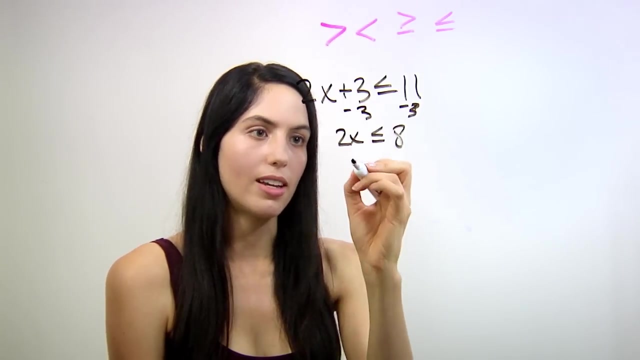 this one. you're going to solve it as you would. an equality, a normal equation. Subtract 3 from both sides So you have 2x is less than or equal to 8.. Divide both sides by 2 so that you have x alone on the left side And you get x is less. 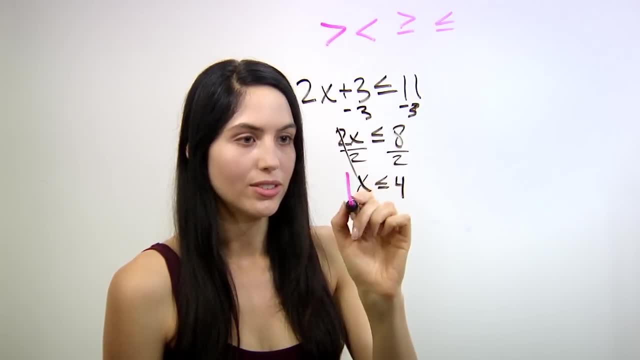 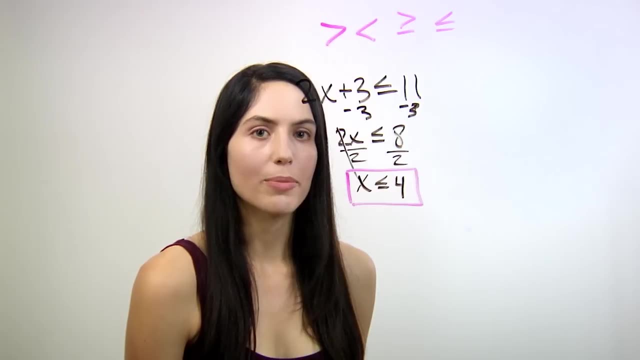 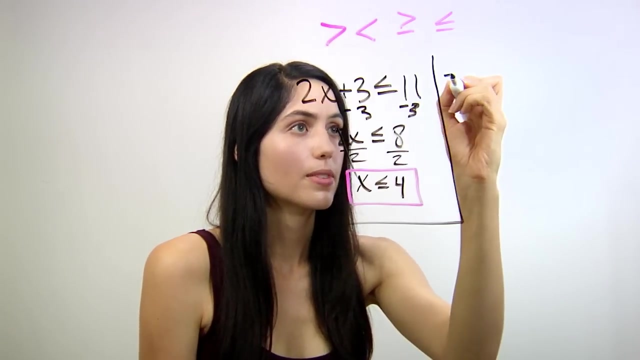 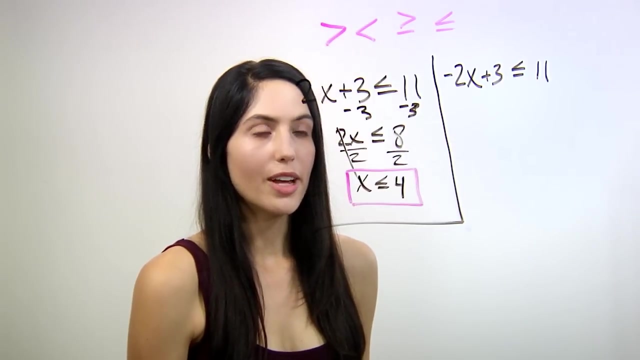 than or equal to 4.. And that's your answer for that simple inequality. Now let's look at a tougher example where it's different from a normal equality equation. Say you have 2x plus 3 is less than or equal to 11.. First step: you do subtract 3 from both sides and 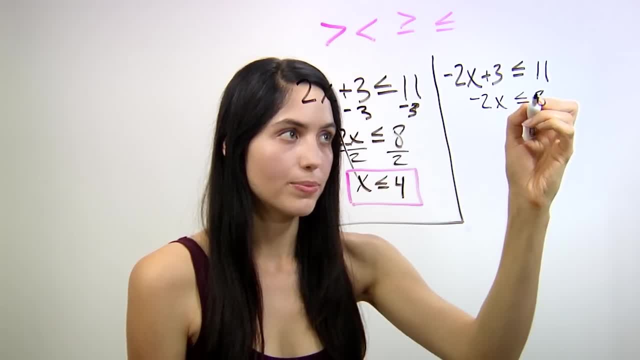 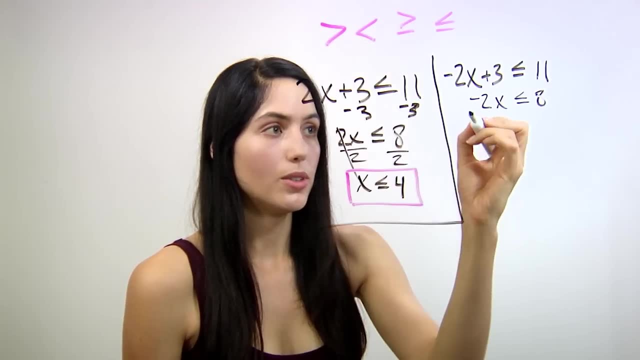 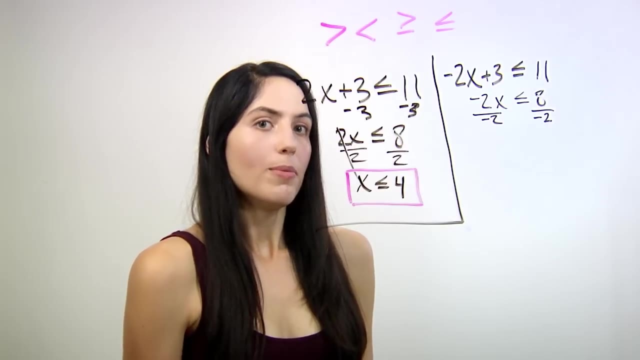 you have negative 2x is less than or equal to 8.. Now you are going to divide out to get x alone. so you would divide by negative 2, divide the right side by negative 2 as well. But here's the trick. 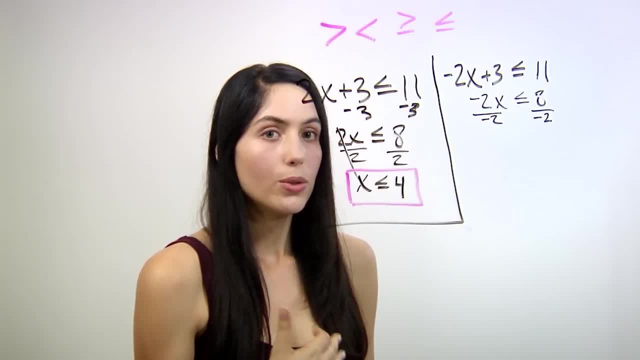 In an inequality you're going to have: 2x plus 3 is less than or equal to 8.. So you're going to have: 2x plus 3 is less than or equal to 8.. And in an inequality if you divide. 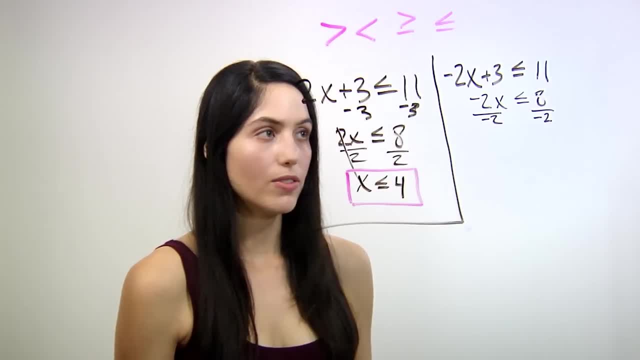 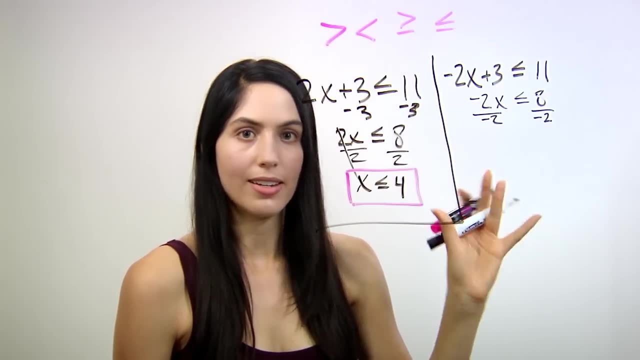 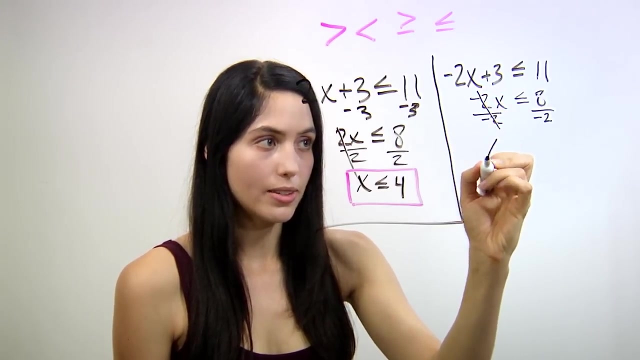 or multiply by a negative number, you have to flip the sign in the middle. You have to flip the direction that your inequality sign faces. So in this equation we divide out negative 2. That goes away. We get x is greater than or equal. to flip the sign negative. 4. 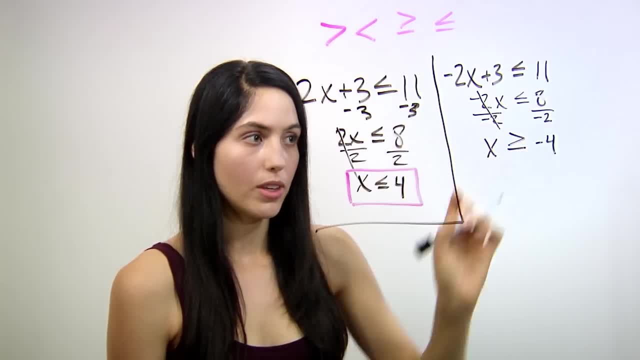 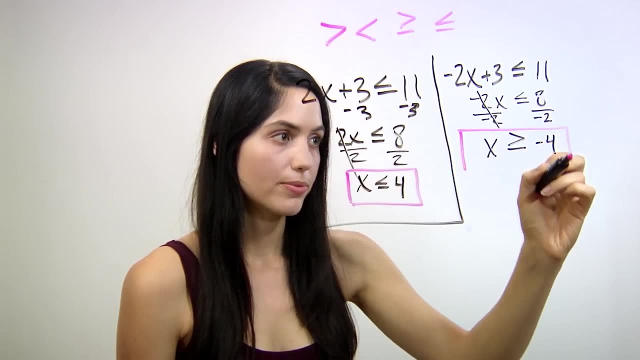 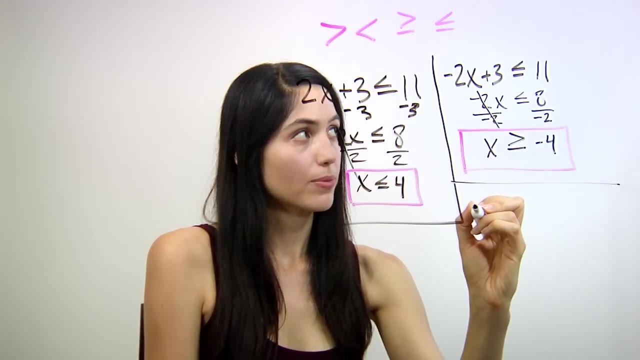 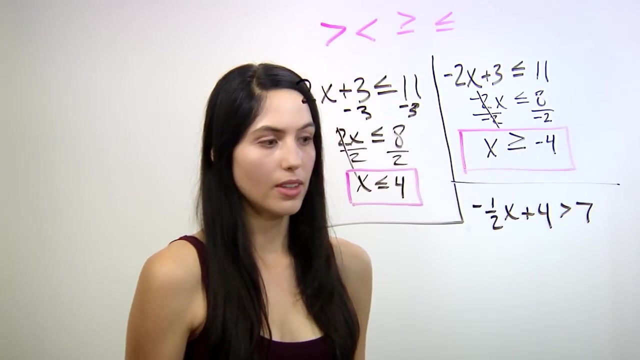 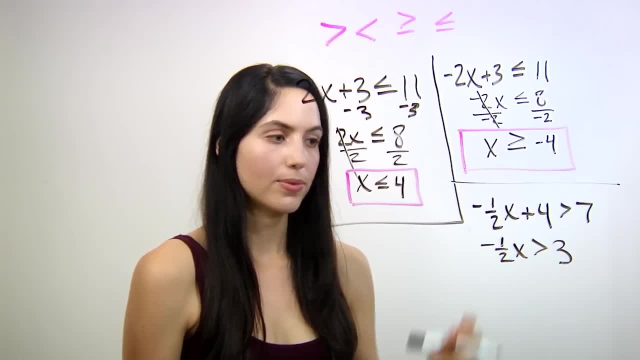 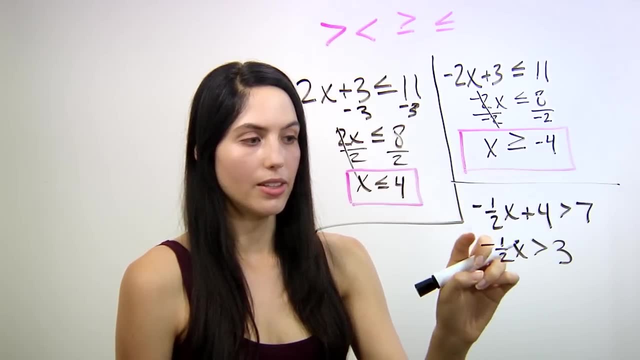 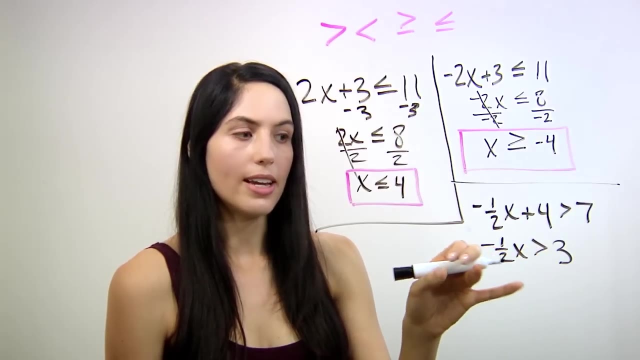 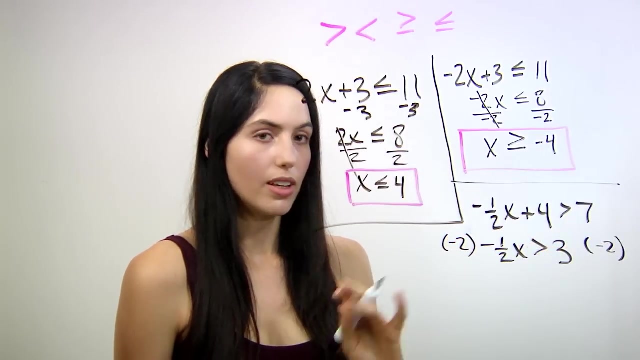 x is greater than 3.. If you want x alone in this equation, you would actually need to clear this fraction, clear the negative 1 half. The fastest way to do that is to multiply both sides by negative 2.. Because if you multiply by negative 2,, 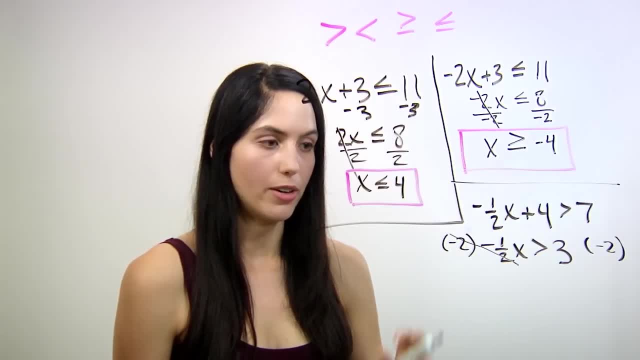 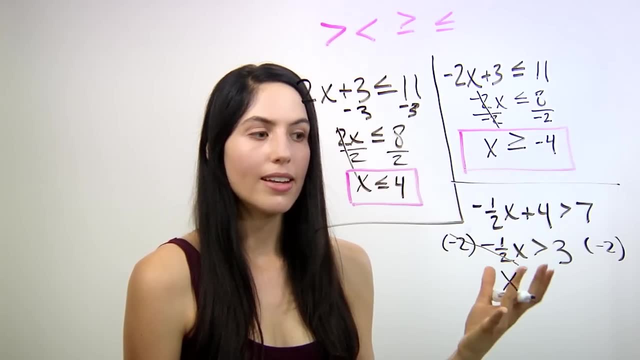 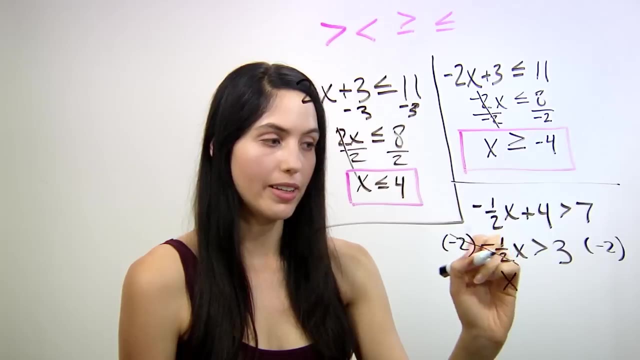 you'll clear the fraction, you'll cancel the 2 in the denominator. Now that would just leave you with x on the left side. but again, because you multiplied by a negative number, you have to flip the direction of the sign, of the inequality sign. 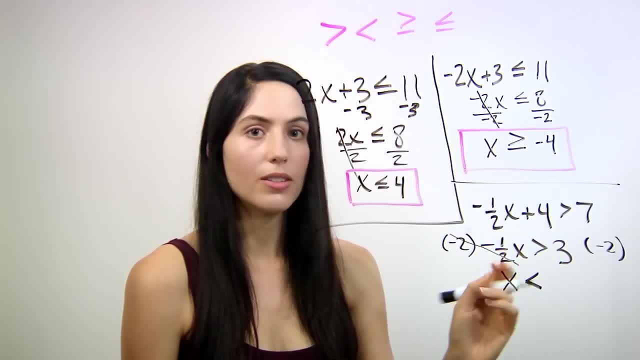 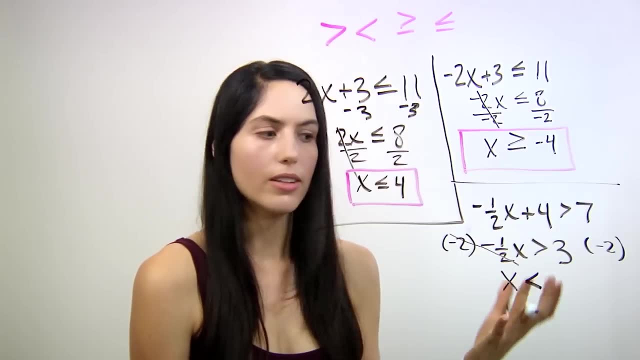 So instead of greater than we now have less than. This is very important because all your other algebra might be correct, but if your sign is flipped you won't get credit. So In this case we have: x is less than negative 6.. 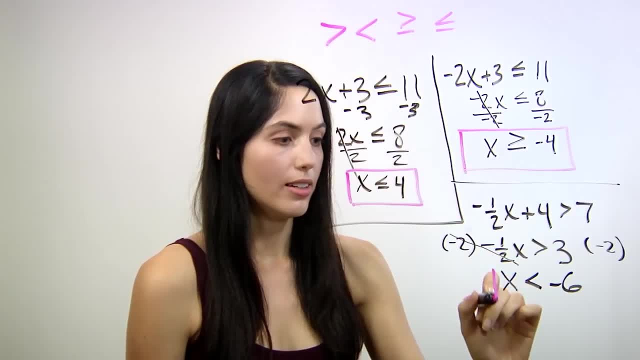 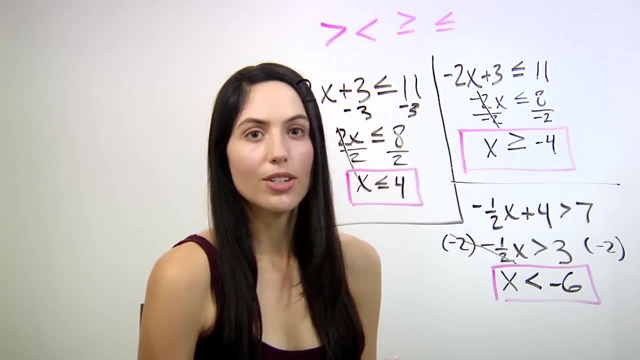 And that's your final answer. x is less than negative 6.. So if you've been having trouble with these inequality problems, just remember it's the same as solving for x in a normal equality, normal equation, except if you ever multiply by a negative number. 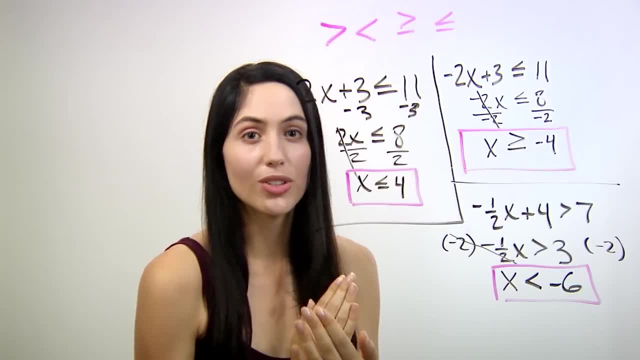 or divide by a negative number, you have to switch the direction of your inequality symbol. You don't have to switch the symbol if you're adding a negative number or subtracting a negative number, only if you're multiplying or dividing by a negative number.